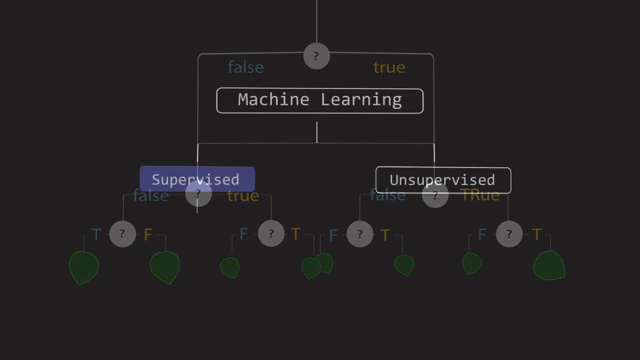 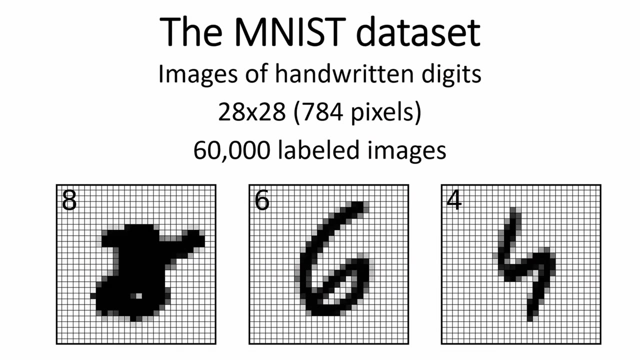 where we talk about the building blocks of these models. In this video, we'll use gradient boosted trees to perform classification. specifically, to identify the number drawn in an image, We'll use MNIST, a large database of handwritten images commonly used in image processing It. 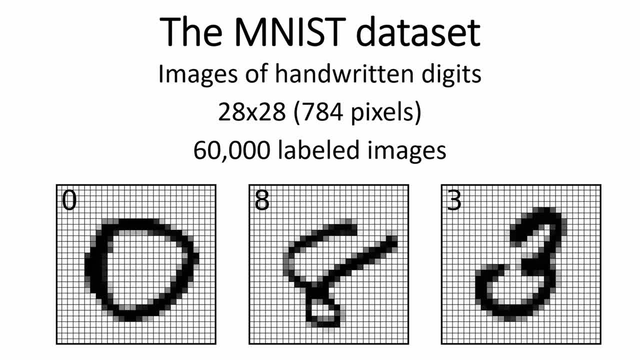 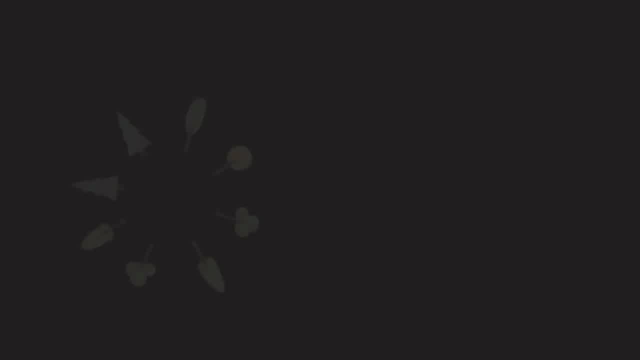 contains 60,000 training images and 10,000 testing images. Each pixel is a feature and there are 10 possible classes. Let's first learn a bit more about the model. Gradient boosted trees and random forests are both ensembling methods that perform regression or classification. 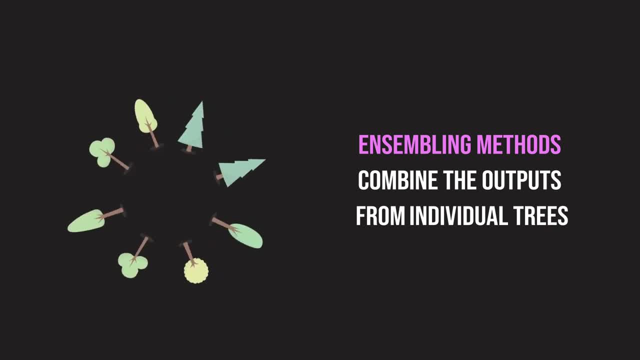 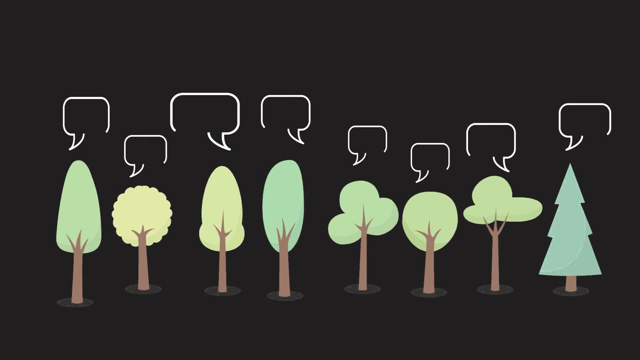 by combining the outputs from individual trees. However, gradient boosted trees and random forests differ in the way the individual trees are built and in the way the results are combined. As you already know, random forests build independent decision trees and combine them in parallel. On the other hand, gradient boosted trees use a method called boosting. 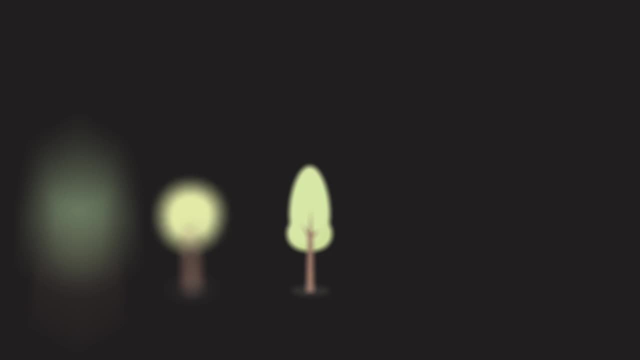 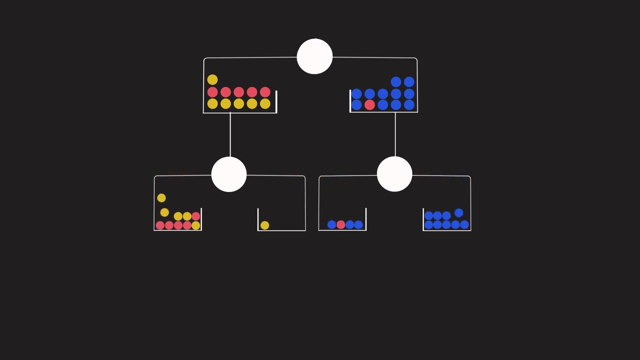 Boosting combines weak learners sequentially so that each new tree corrects the errors of the previous one. Weak learners are usually decision trees with only one split called decision stumps. So the first step is to fit a single decision tree. We'll evaluate how well this tree does using a loss function. There are many different loss. 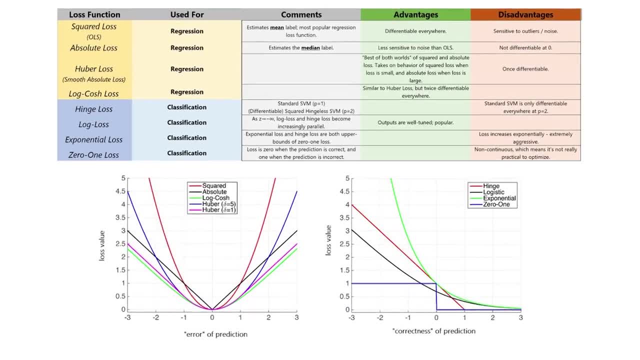 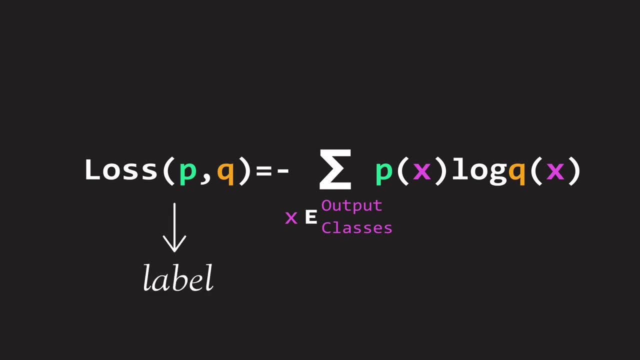 functions we can choose from. For multi-class classification, cross entropy is a popular choice. Here's the equation for cross entropy, where p is the label and q is the prediction. Basically, the loss is high when the label and prediction do not agree. 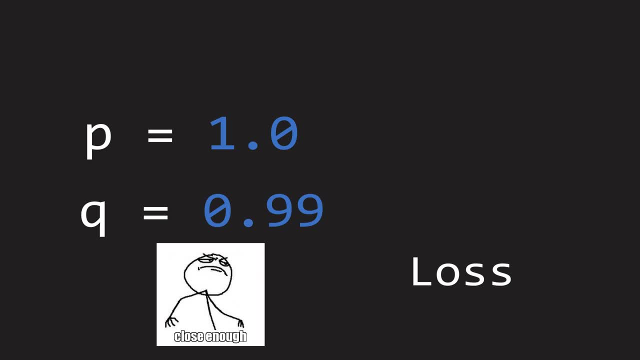 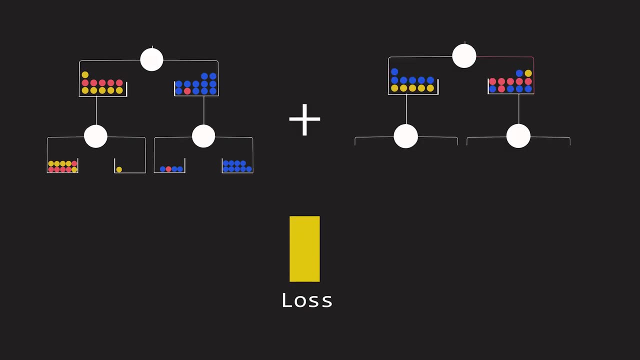 and the loss is zero when they're in perfect agreement. Now that we have our first tree and the loss function we'll use to evaluate the model, let's add in a second tree. We want the second tree to be such that, when added to the first, 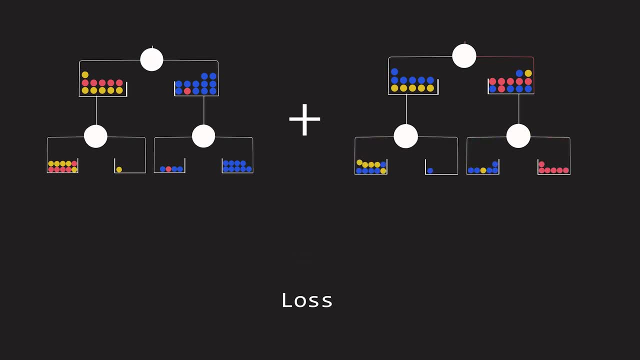 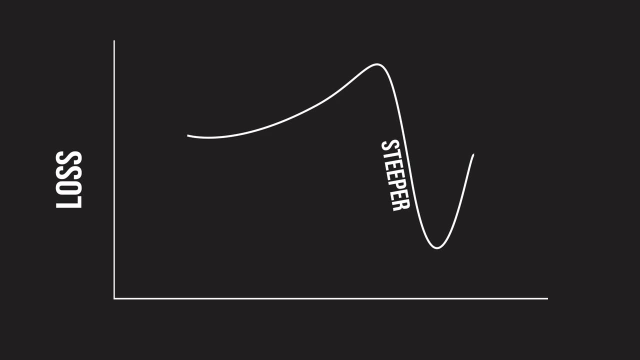 it lowers the loss compared to the first tree alone. Here's what that looks like. where eta is the learning rate. We want to find the direction in which the loss decreases the fastest. Mathematically, this is given by the negative derivative of.